Would you please send Jake Swisher to the front office to check out, please? 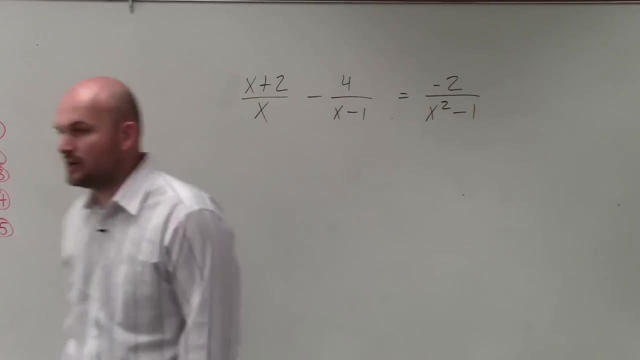 Okay. Just make sure you write down your homework, okay? And I'll put this online as well. 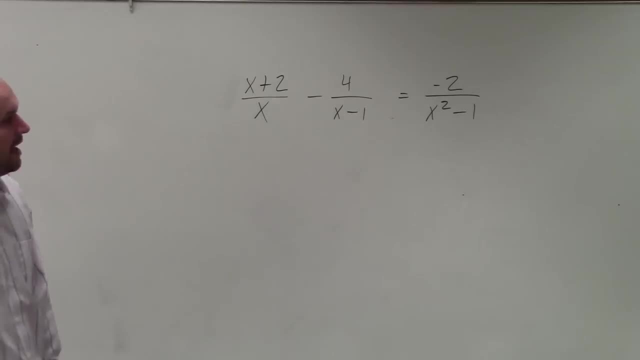 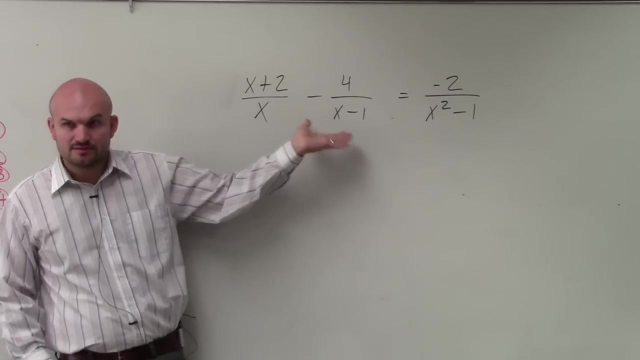 So, ladies and gentlemen, when you're looking at a problem like this, do you guys remember the problems that we wrote down last class period? Where I saw, it was basic fractions, but we had like a variable in the denominator, right? You guys remember that? Okay. 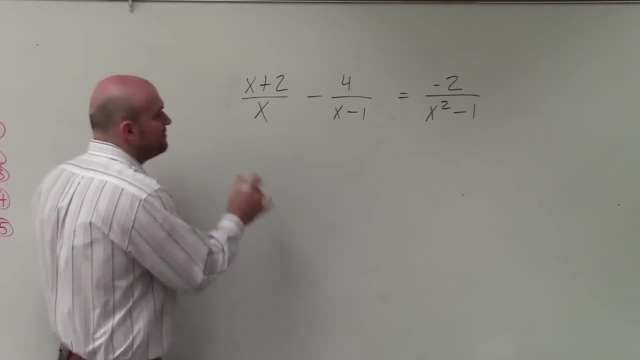 Okay. So, the main important thing, whenever you're solving, the main thing we got to do is get these variables off the denominator. 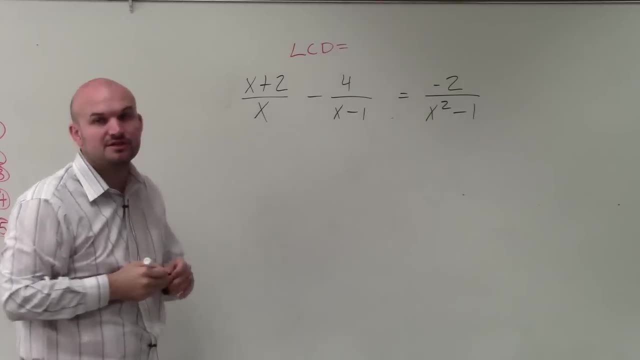 So, to do that, what we're going to want to do is multiply every single term by the LCD. So, we have to figure out what the LCD is. 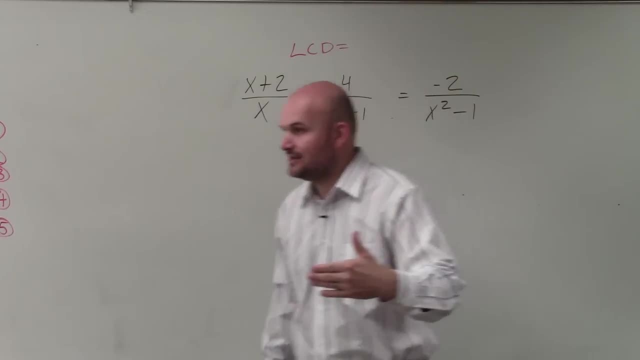 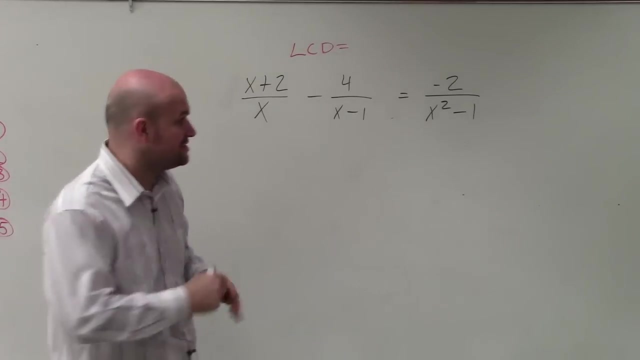 Now, in our focus lessons, we practiced... Remember when we were adding and subtracting, right? With unlike denominators, we had to find the LCD. Or when we were doing complex fractions, basically what we did was multiply everything by the LCD, which is the same thing. 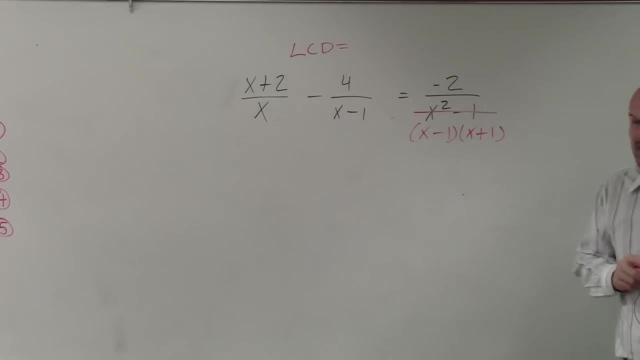 So, the first thing we want to do is factor anything that we can. Always factor. That's going to be simplifying this. 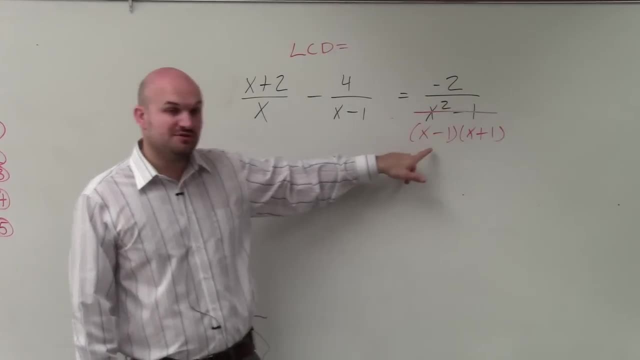 So, now you guys see, x squared minus 1, I factored using difference of two squares as x minus 1, x plus 1, okay? 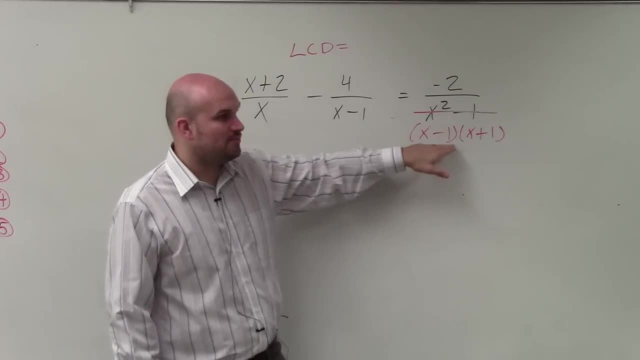 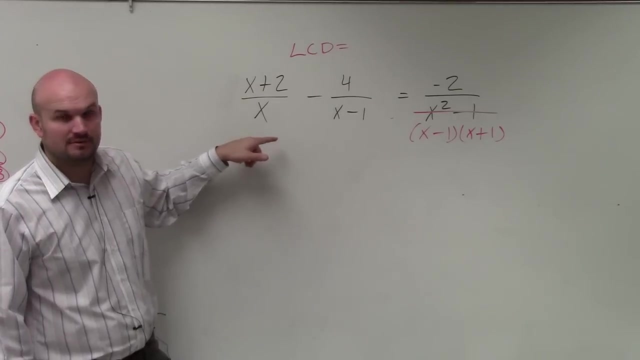 So, now I need to find the polynomial that both x minus 1 and x plus 1 and x all divide into. Agreed? Okay. So, my LCD. Okay. 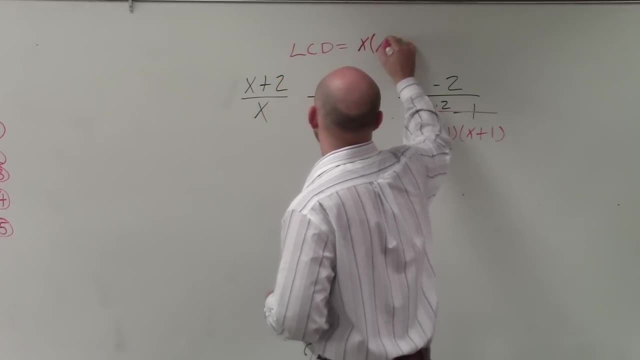 My LCD is going to be x times x minus 1 times x plus 1. 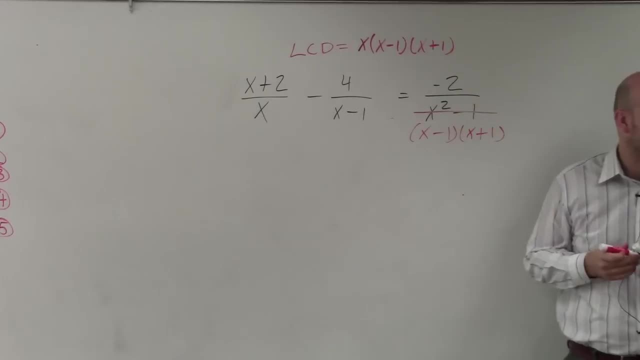 Do you guys agree with me that every single one of my denominators divides into that LCD? Yes? Okay. 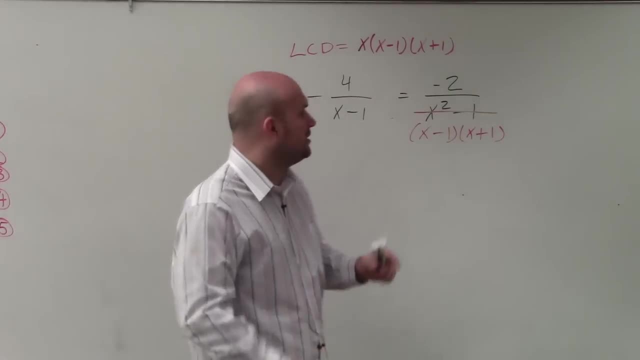 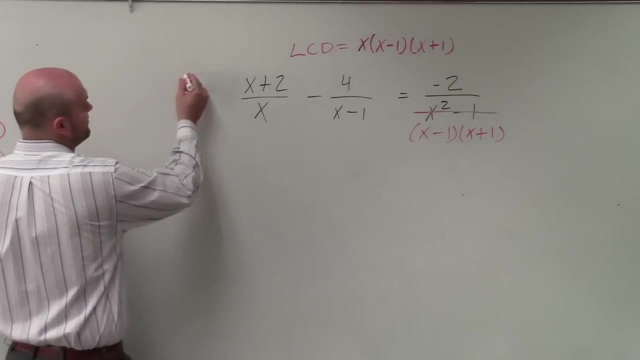 So, now, how do we use that LCD to help us solve? Well, if we multiply every single one of our terms by our LCD, we can use the division property to simplify. So, what I simply do is just write it multiplication times every single term. All right. See ya. 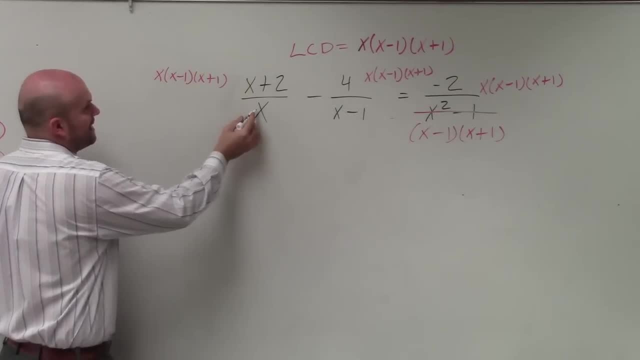 So, let's see what happens using the division property. X divided by x. That divides out. 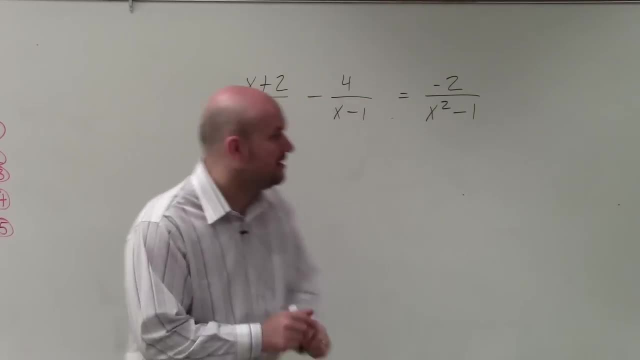 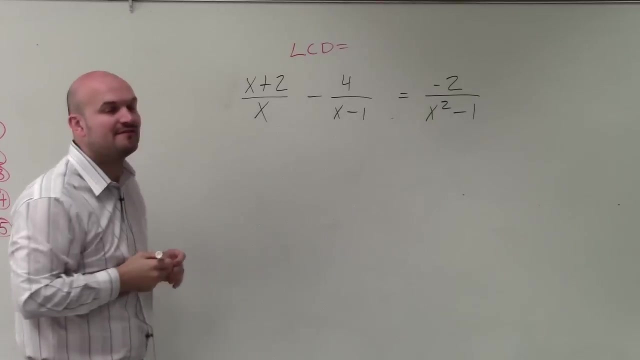 You guys remember that, Okay, Okay. So the main important thing whenever you're solving, the main thing we got to do is get these variables off the denominator. So to do that, what we're going to want to do is multiply every single term by the LCD. 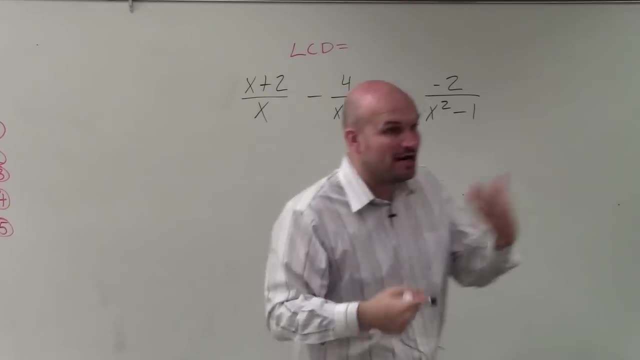 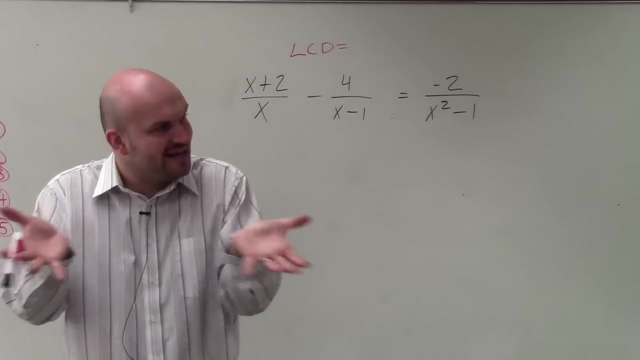 So we have to figure out what the LCD is Now. in our focus lessons we practiced- Remember, when we were adding and subtracting right With unlike denominators, we had to find the LCD. Or when we were doing complex fractions. 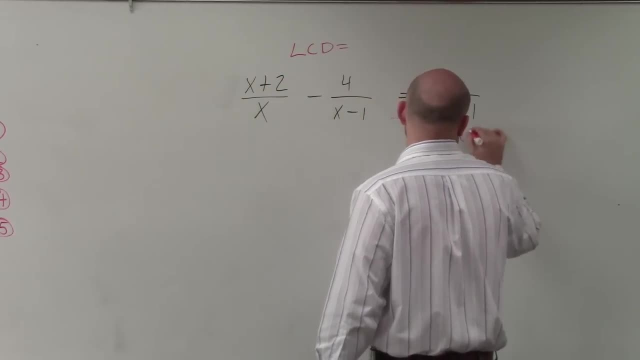 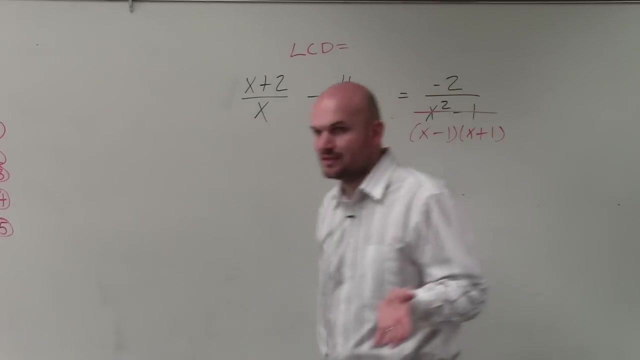 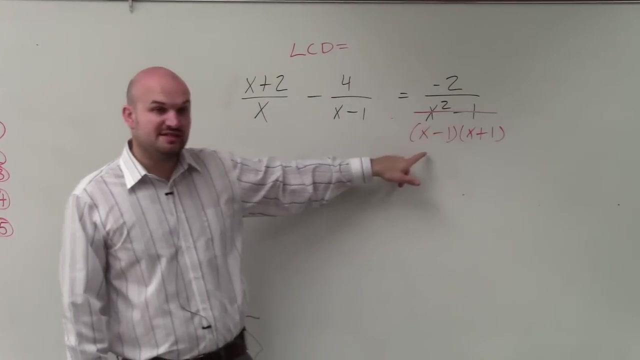 basically, what we did was multiply everything by the LCD, which is the same thing. So the first thing we want to do is factor anything that we can Always factor. That's going to be simplifying this. So now you guys see x squared minus 1, I factored using difference. 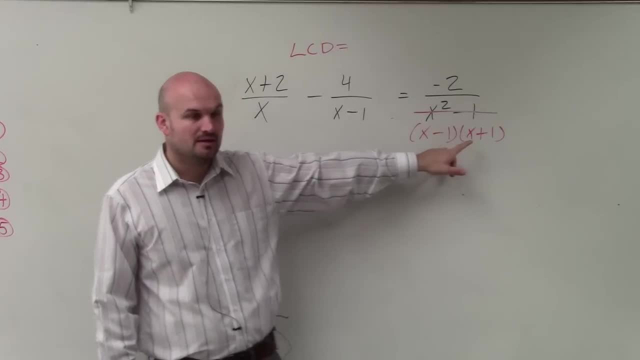 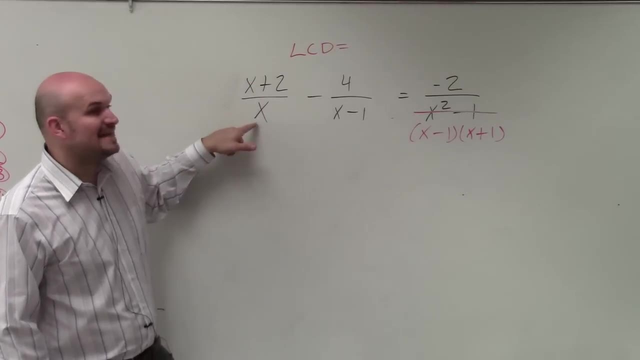 of two squares as x minus 1, x plus 1, okay, So now I need to find the polynomial that both x minus 1 and x plus 1 and x all divide into Agreed. Okay, So my LCD. 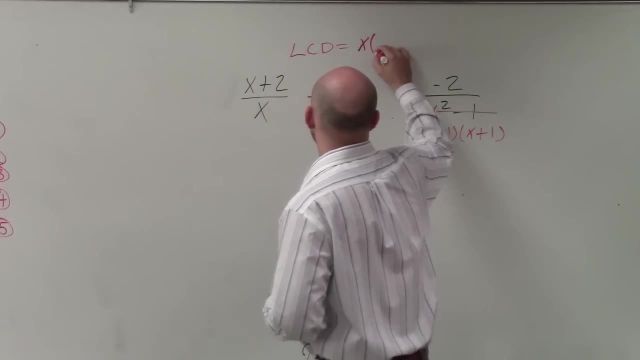 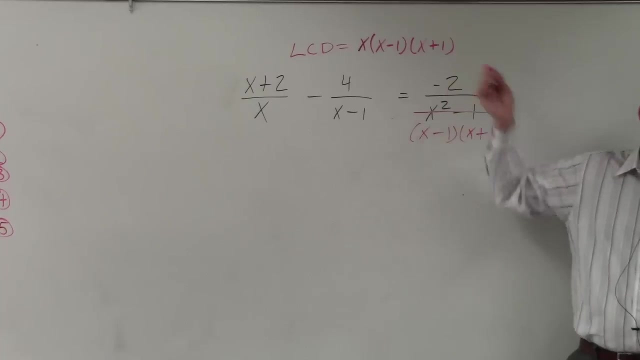 Okay, My LCD is going to be x times x minus 1 times x plus 1.. Do you guys agree with me that every single one of my denominators divides into that LCD? Yes, Okay. So now how do we use that LCD to help us solve? 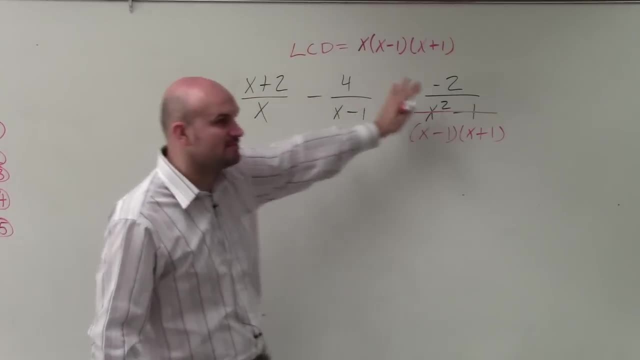 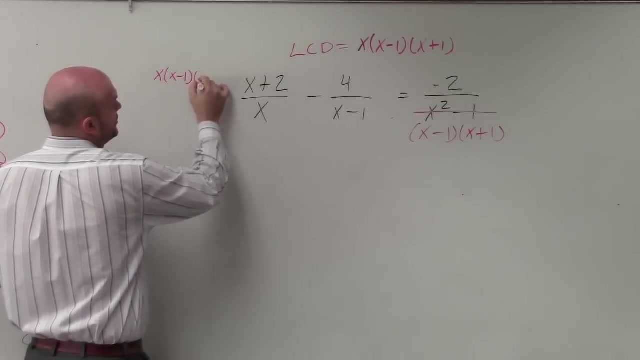 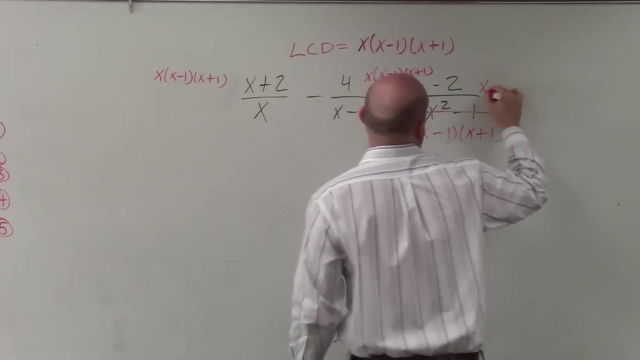 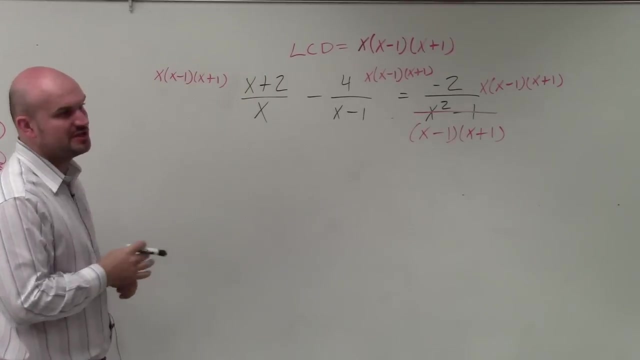 Well, if we multiply every single one of our terms by our LCD, we can use the division property to simplify. So what I simply do is just write it: multiplication times every single term. Alright, see ya. So let's see what happens using the division property. 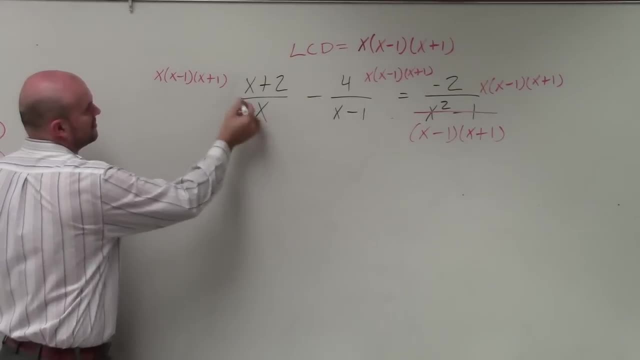 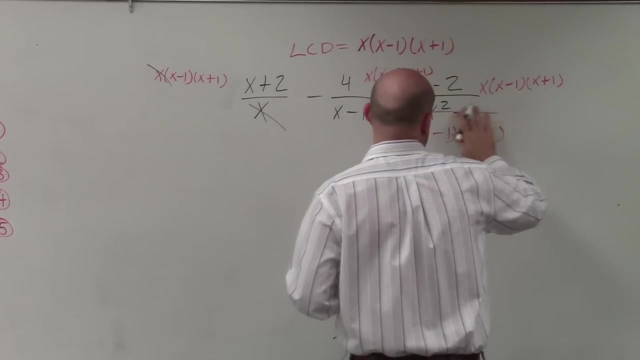 x divided by x, That divides out Whoa, whoa, whoa, whoa, whoa, whoa. Oh, I'm an idiot, I wrote the wrong problem down. I'm sorry. Sorry about this, Hold on Sorry. 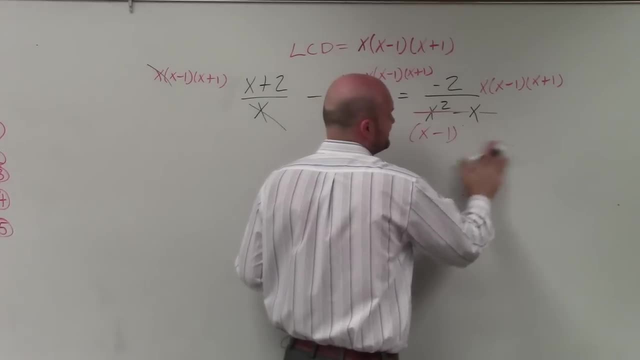 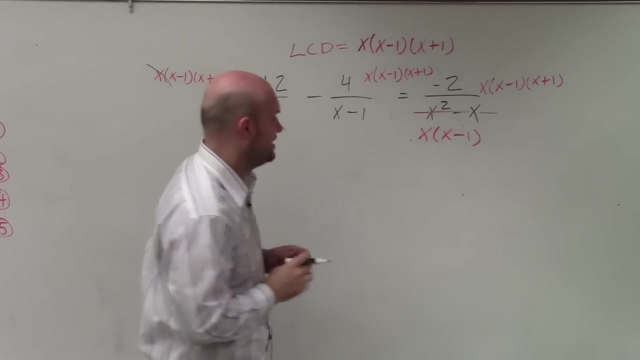 This problem was x squared minus x, Sorry, So therefore this gets factored into x times x minus 1.. Sorry, I don't want to over-make this problem, I just realize I'm like this is going to be an issue. Whoa, whoa, whoa, whoa, whoa, whoa. Oh, I'm an idiot. I wrote the wrong problem down. I'm sorry. Sorry about this. Hold on. Sorry. This problem was x squared minus x. Sorry. 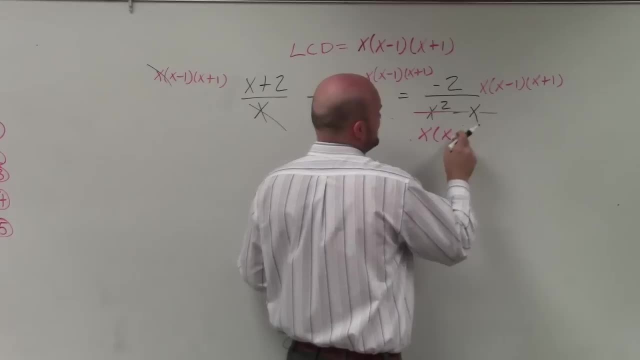 So therefore, this gets factored into x times x minus 1. Sorry. 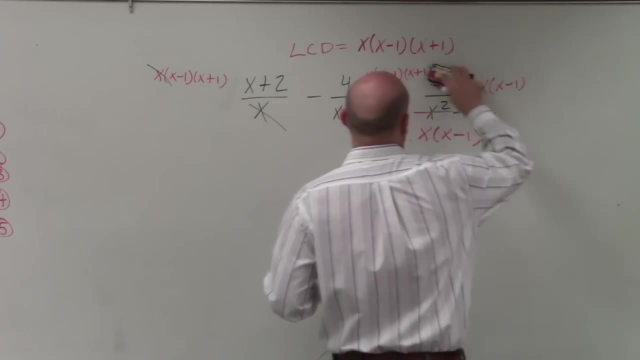 I don't want to over make this problem. I just realize I'm like, this is going to be an issue. We're going to have a cubic. 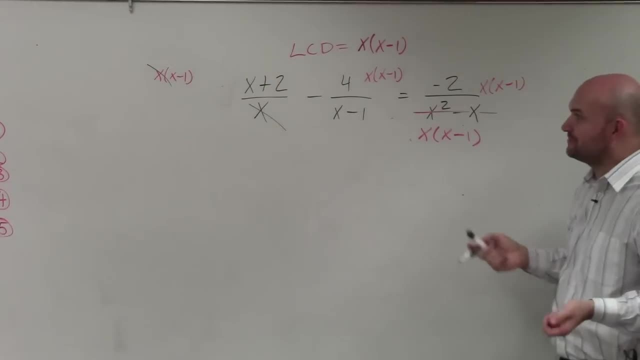 And not like you couldn't do it, but that's just going to make this problem much more difficult. 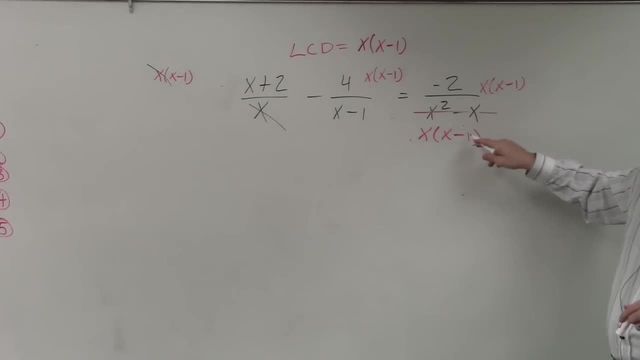 So anyways, this gets factored down to x times x minus 1. Therefore, my LCD is x and x minus 1. Does that make sense? OK. OK. 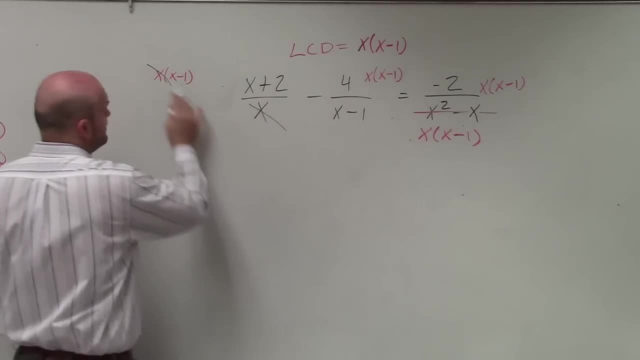 So if I multiply everything times x times x minus 1, my x's divide out. Here, my x minus 1's divide out. 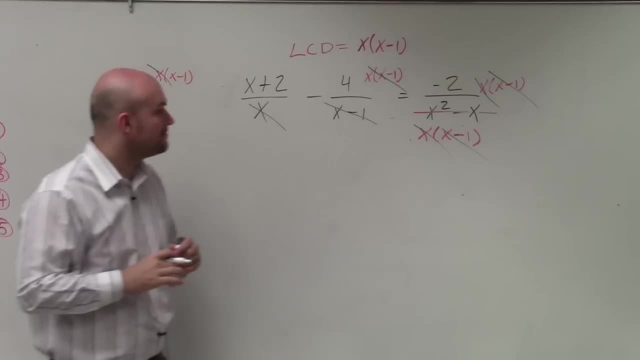 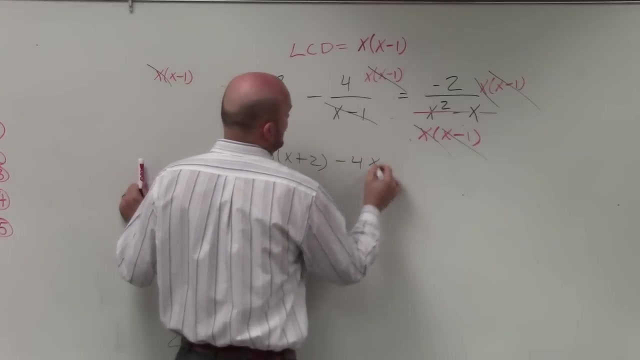 And here, my x's and the x minus 1's divide out to 1. So therefore, now I'm left with an x minus 1 times x plus 2 minus 4 times x. Equal. Negative 2. Does everybody follow me? Anybody have any questions? Are we OK? I'm just waiting for questions. We're good. Kind of. 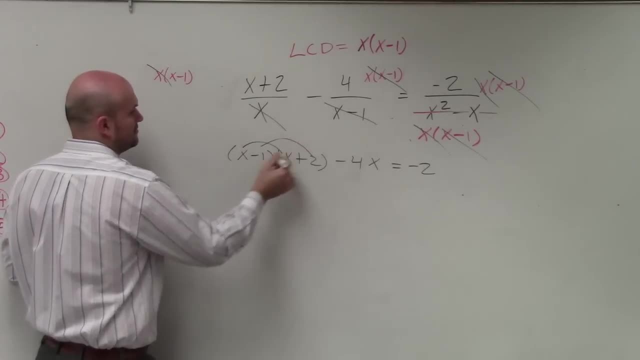 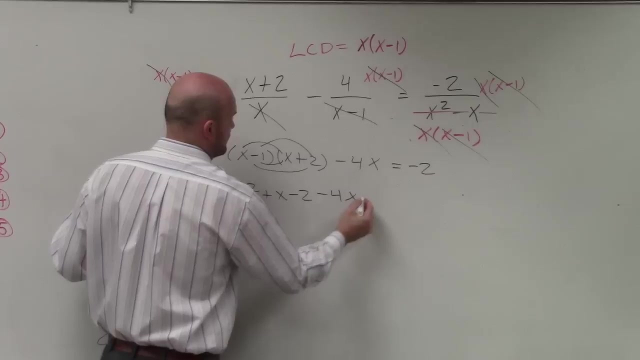 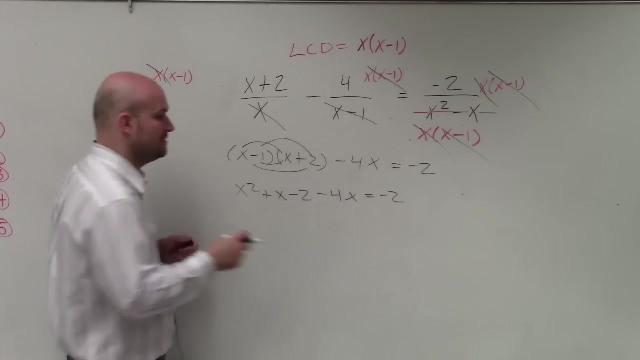 Now, apply FOIL here. You get x squared plus x minus 2. Minus 4x equals negative 2. I realize this is a quadratic. So I'm going to get all my terms onto the same side. Right? So I'll add a 2. 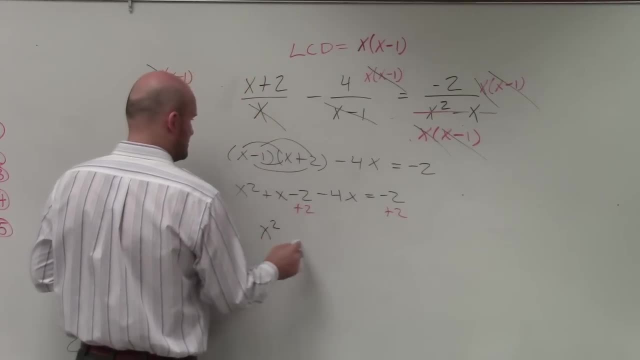 Add a 2. And I get x squared, let's see, minus 3x equals 0. Now, yes? 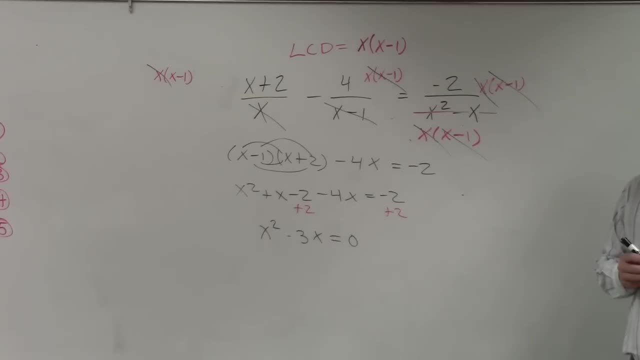 When you have the 4 up there, it has to be 4 plus x. Yeah. Yeah. Well, the x minus 1 is divided out. So that's x. Now, remember, what am I doing with this LCD? I'm multiplying the LCDs, right? So that's really 4 times x. OK. Does everybody follow me so far? 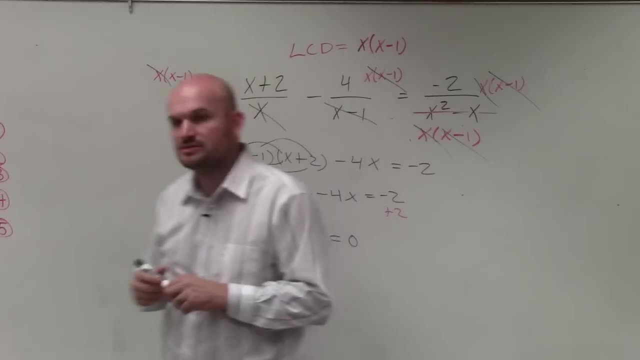 Anybody have any other questions? 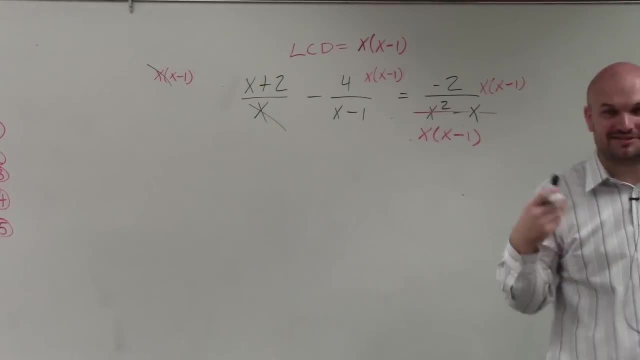 We're going to have a cubic, And not like you couldn't do it, but that's just going to make this problem much more difficult, Cool, So anyways, this gets factored down to x times x minus 1.. Therefore, my LCD is x and x minus 1.. Does that make sense? 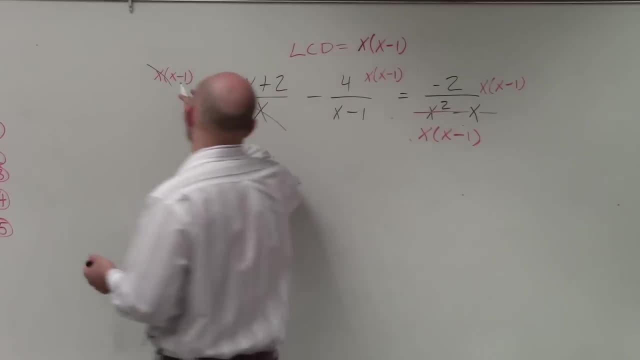 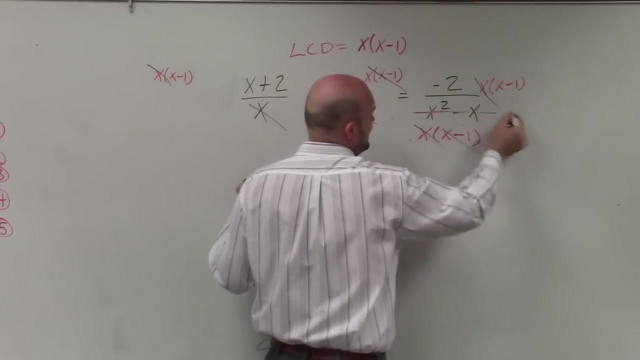 Okay, So if I multiply everything times x, times x minus 1, my x's divide out, Here my x minus 1's divide out, And here my x's and the x minus 1's divide out to 1.. 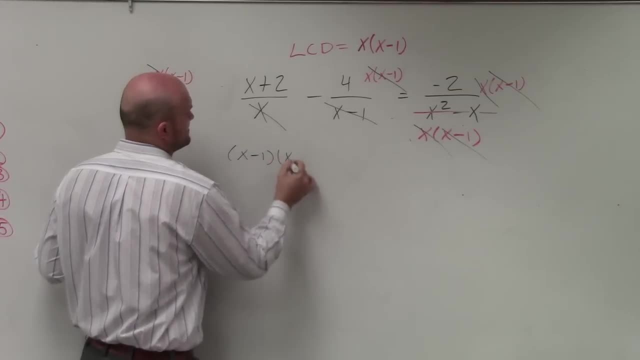 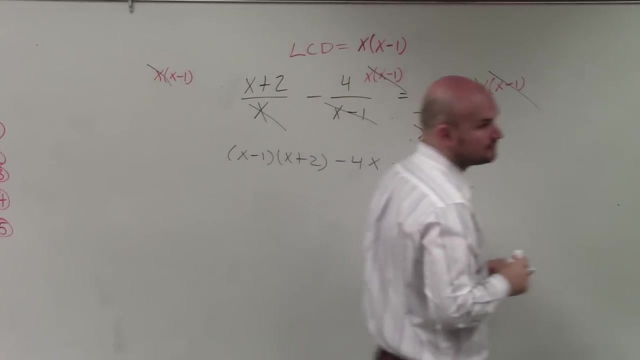 So therefore, now I'm left with an x minus 1 times x, plus 2 minus 4 times x equals, equals negative 2.. Does everybody follow me? Anybody have any questions? Are we okay? I'm just waiting for questions. 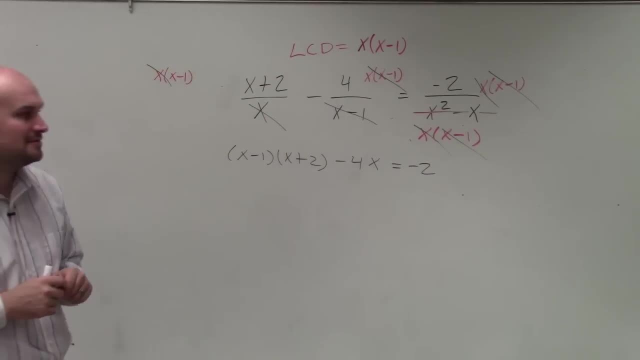 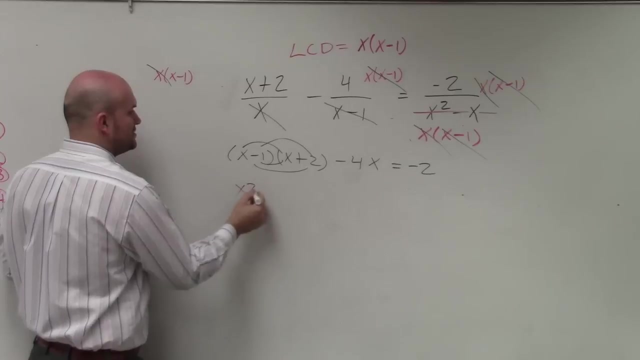 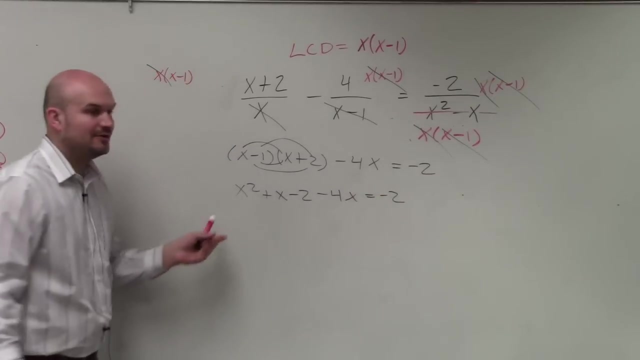 We're good. Kind of Now apply FOIL here You get x squared plus x minus 2.. Minus 4x equals negative 2.. I realize this is a quadratic, so I'm going to get all my terms onto the same side, right? 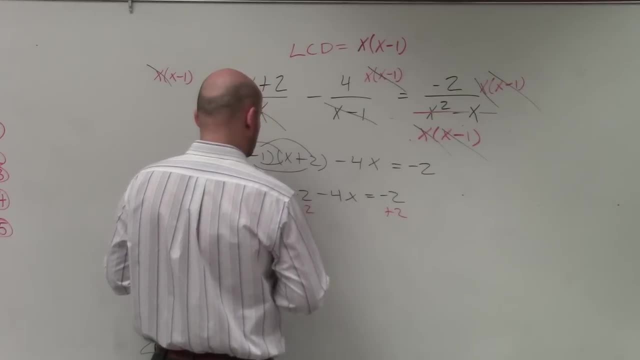 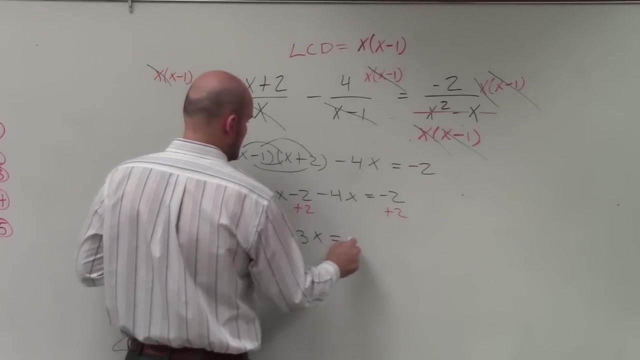 So I'll add a 2.. Add a 2. And I get x squared. let's see: minus 3x equals 0.. Now, yes, Yes, When you have the 4 up there, how do you form the x? 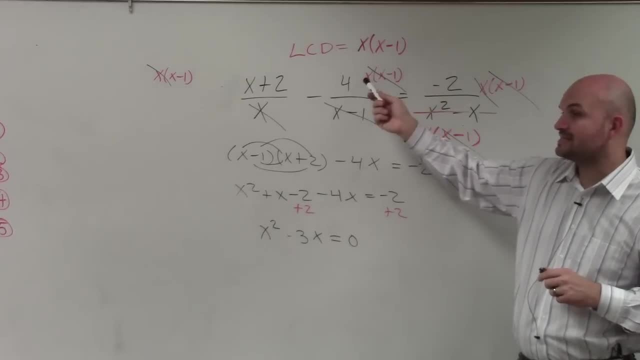 Well, the x minus 1's divided out, so that's x. Now, remember what am I doing with this LCD? I'm multiplying the LCDs, right? So that's really 4 times x. Okay, Has everybody followed me so far? 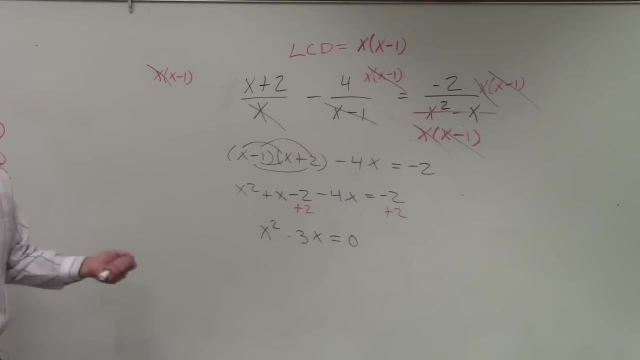 Anybody have any other questions? Now, yes, What is this called Like? what is this? I mean, We're just multiplying by the LCD. We're solving rational equations. That was. It's the same topic that I started with last class period, so that's why I didn't write it. 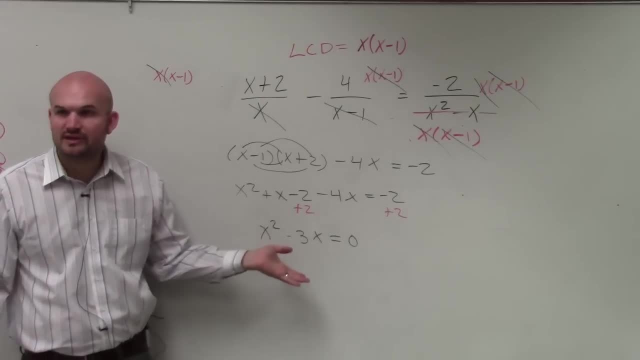 So that's why I didn't write it up there. Now, in this case, we don't really actually have to factor using a trinomial or quadratic formula. This one's actually not that bad. I can just factor out the x.